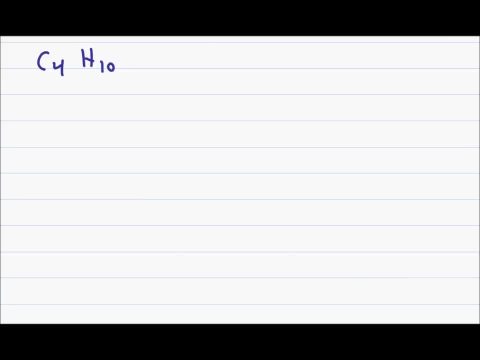 difference between something that is an isomer and something that is drawn in the same way. For example, we had a straight chain written out. but what if I decide to try an isomer that looks something like this: In line structure that would look like a straight chain or one with a bend. 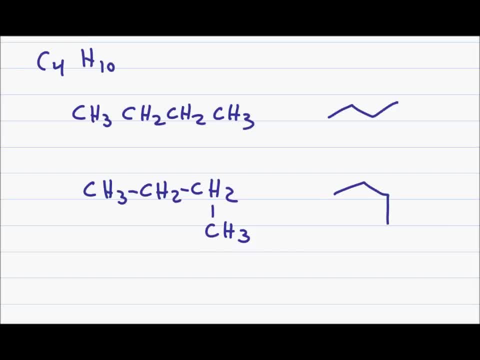 chain. While looking at it, it appears to be different. These two are actually the same exact molecule. So how do you tell the difference? Simple, Just name your molecule. So I will start by numbering this one and notice that I can number. 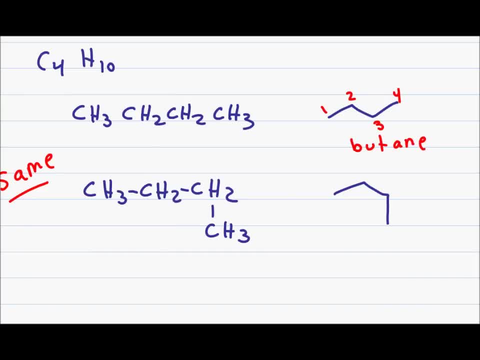 four carbons in a row, which gives me a butane, And for the second one, when I number it once again, I get four carbons in a row for butane. so I know it's the same thing. One more thing to. 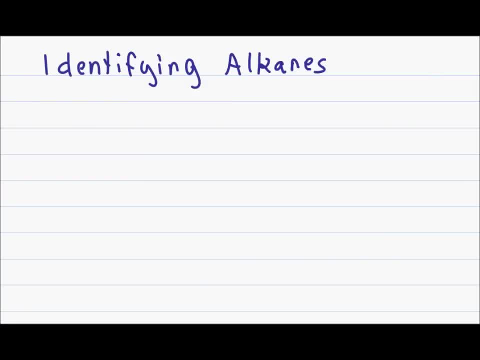 consider before doing these problems. I said this video will be about alkanes but say: you're not sure, How do you know that the molecule in question is an alkane? Recall that the formula for an alkyl- the formula for an alkane is CnH2n plus two. This means that if I have n number of carbons, then the 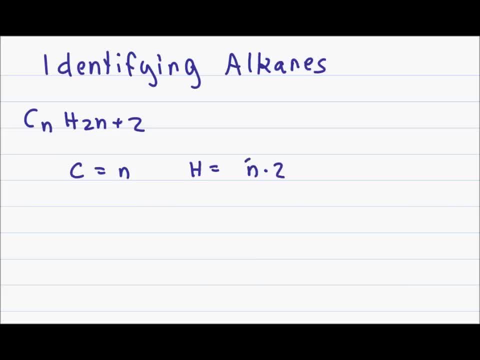 hydrogens will be the number of carbons times two plus two. Going back to my previous formula, we had C4H10.. If C is equal to four, that means I have four carbons. To find the hydrogen number, that's n. 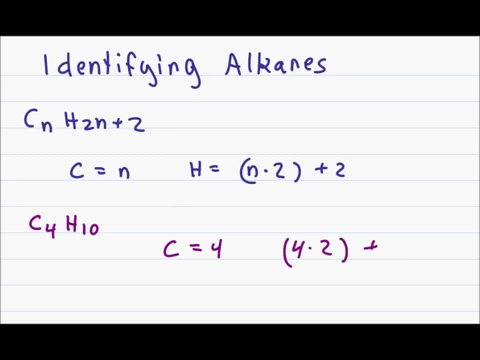 times two, meaning four times two plus two, That's eight plus two, which is ten, and that means I have ten hydrogens in my formula for an alkane. What happens when you have less than ten hydrogens? That's when we get into the concept of 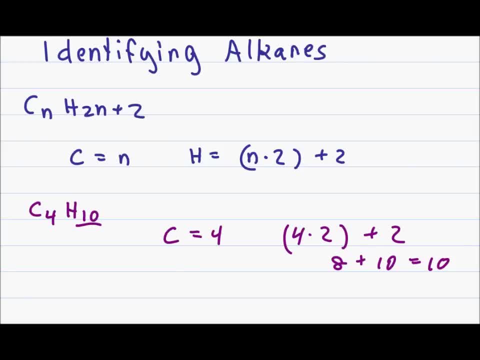 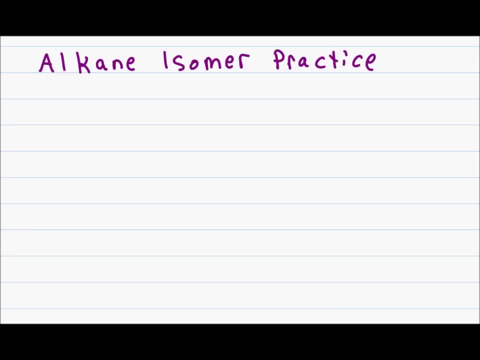 hydrogen deficiency and pi bonds and rings, which will be addressed in my next video on constitutional isomers. Let's try some practice problems. We'll start with a rather simple example- C5H12, and let's see how many isomers we can come up with. 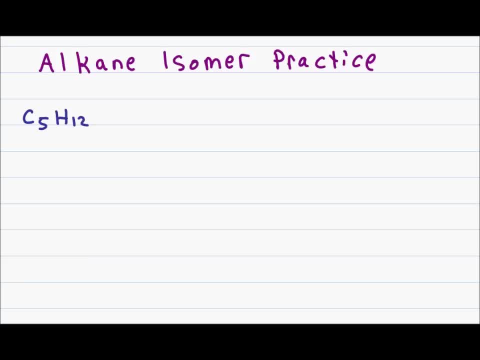 If you're not sure, if a molecule is the same name the molecule, If the name is the same, then it's the same. Carbon is five. that means hydrogens should be two times five plus two, which is ten plus two is twelve and we. 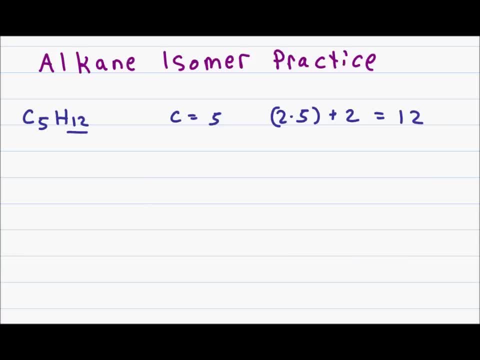 know we have an alkane. The trick to finding all or most of the isomers is to work methodically rather than randomly writing what comes to mind. The way to do this is starting with a straight chain and then slowly shortening your chain, adding branches and then adding more branches. 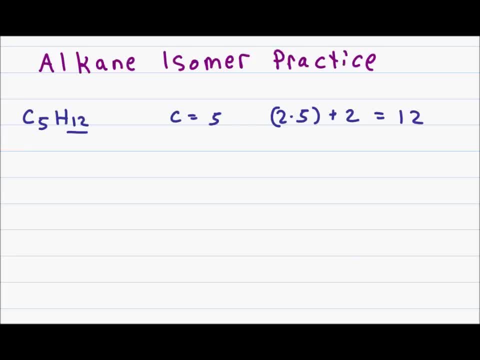 And moving them from one side of the molecule to the other. The first structure that comes to mind, obviously, is the straight chain of five carbons. There are no substituents to move around, so that's the only five carbon straight chain isomer. The next isomer is going to have four carbons with one. 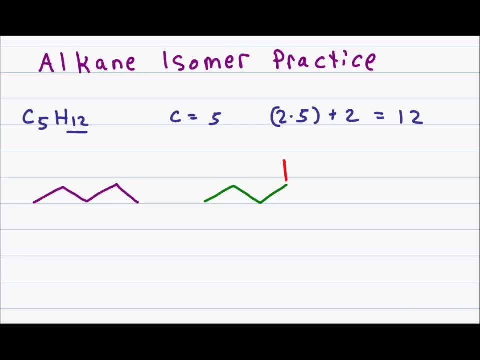 methyl substituent. If I put the substituent on carbon one and I name it, I have pentane for my substituent, but this is the same thing. Instead, I will put the substituent on carbon number two. Now, when I name it, my parent chain only has four carbons and I have a methyl substituent giving me two methylbutane. 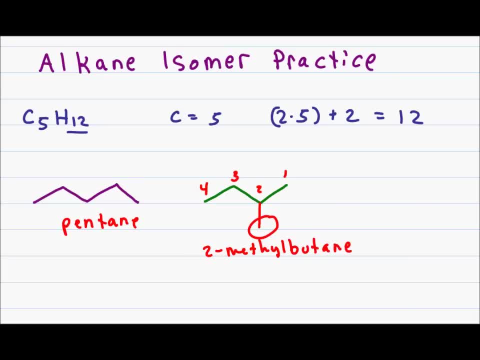 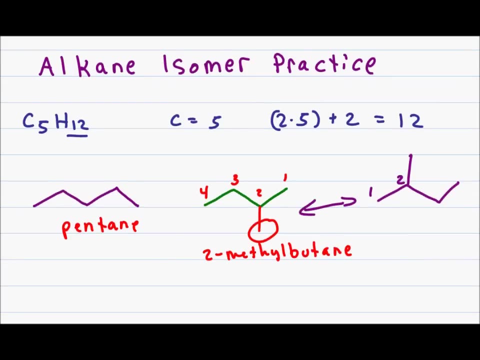 If I take this substituent and move it to carbon number three, it's actually just two methylbutane in reverse, because I number it from the side that reaches the substituent First and once again I get two methylbutane. So that's all I have for one branch on a four carbon chain. 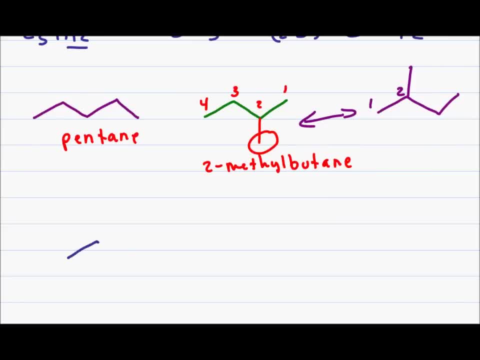 Now let's try a three carbon chain For three carbons. the only place to put two methyl substituents is on the center carbon Numbering it. I have a parent chain of three with two methyls on carbon two. This gives me. 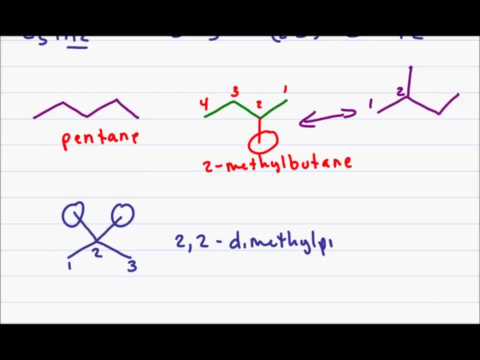 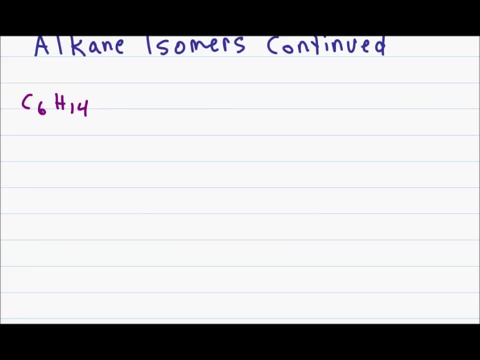 2,2-dimethylpropane. Working our way up, let's try C6H2O. The good news about these molecules is that as you increase the number of carbons, you increase the possible isomers, And professors will usually ask you to find the majority, but not every single isomer, so it's okay to miss one. 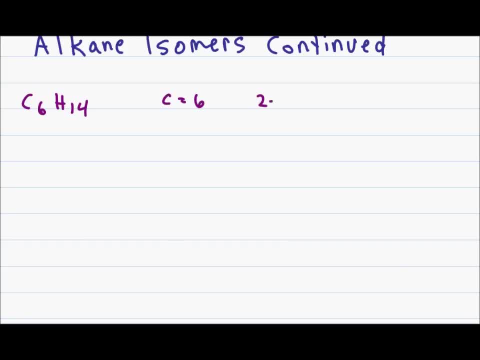 Carbons, we have six. That means hydrogens will be two times six, which is twelve plus two. fourteen: We have fourteen hydrogens. We have an alkane. I will start with a straight chain of six carbons, giving me hexane. 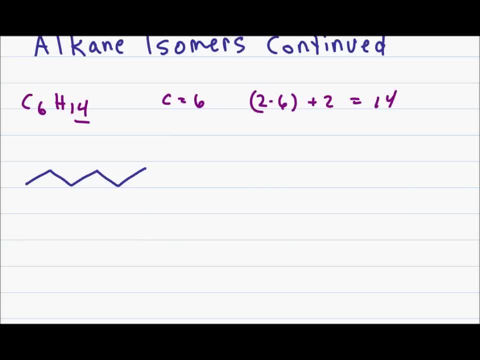 And then move onto branching. In this case, I actually have the opportunity to move my branches around. If I have five carbons, I can put the methyl substituent in multiple places. Putting a methyl substituent on carbon one will just give me another hexane, so that's no good. 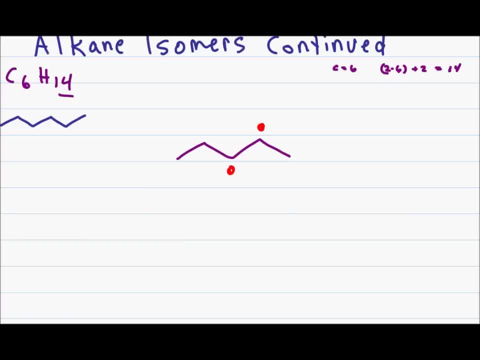 I can put a substituent on carbon two and carbon three. If I put it on carbon four, that's really just two from the other side, and carbon five is just one from the other side. I will draw my two 5-carbon chains with a methyl substituent and then name it, just to. 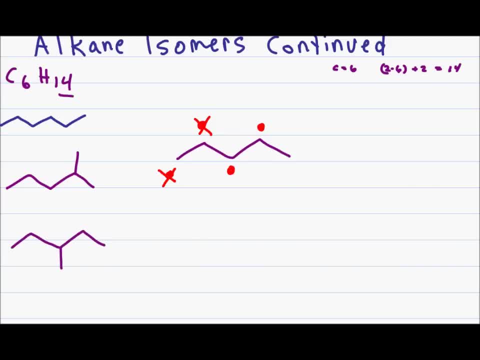 make sure that they're not the same molecule. For the first one, I have 2-methylpentane, and for the second one, I have 3-methylpentane. Next I move on to a 4-carbon chain and, in order to reach C6, I have two methyl substituents. 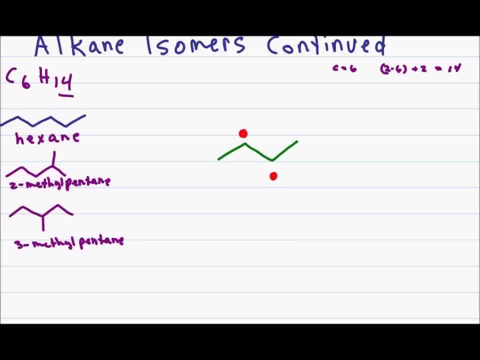 I have the option to place one on carbon 2 and one on carbon 3, or I can place two substituents on the same carbon. For the first one, I have 2, 3-dimethylbutane. then I can do 2, 2-dimethylbutane. 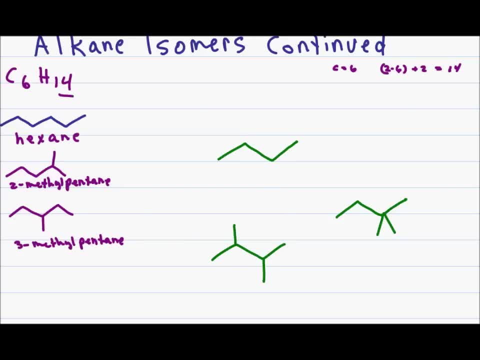 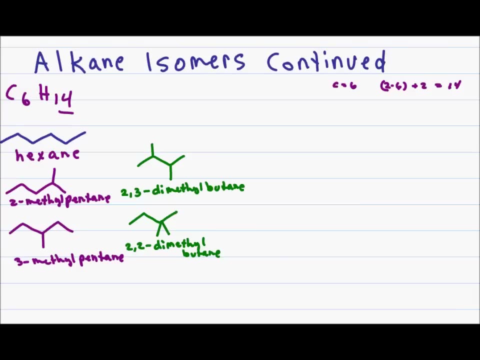 Now be careful not to do a butane with an ethyl substituent, because if you number this, you actually get a 5-carbon chain with one methyl substituent, which is the same as your 3-methylpentane. Removing another carbon from the parent chain would give me three carbons. 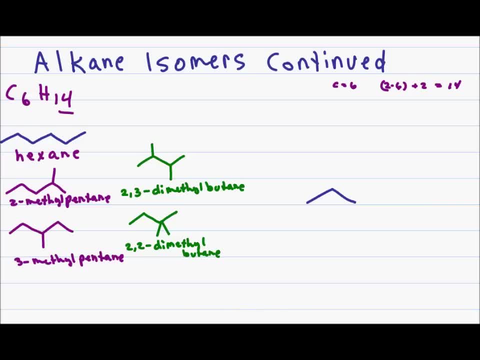 In this case, however, I need three methyl substituents in order to have six carbons, and since I can only place two on the center carbon, I would have to put my third carbon on a carbon. that would increase the length of the chain. 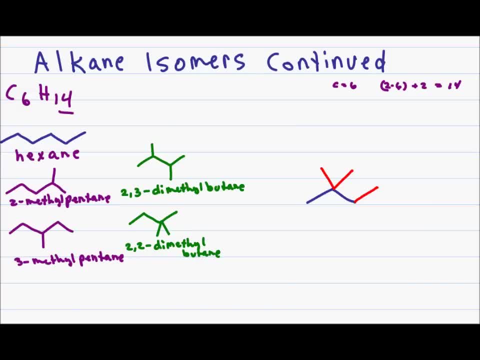 In this case, I have 2,2-dimethylbutane, which we already have, If I put it on the substituent itself. I now have one, two, three, four, again 2,2-dimethylbutane. 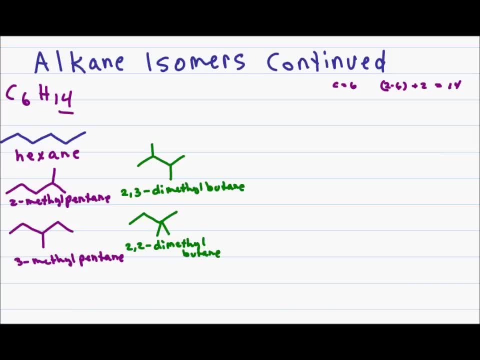 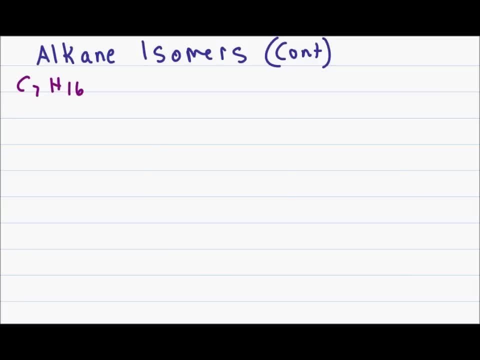 So for C6H14, we have a total of five isomers. Now let's try C7H16.. Remember, as the number of carbons goes up, the number of isomers go up. so just be careful, Try to get as many as you can. 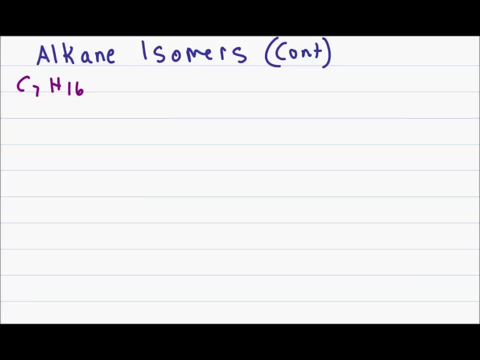 And name them, to make sure you don't have duplicates. I won't be naming them as I draw them, otherwise they would fill the screen And if I miss one or two, please don't hold it against me. There are a couple. 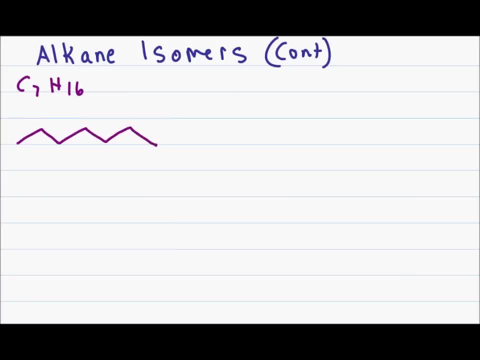 I will start with the straight chain of seven carbons, and this is heptane. For the 6-carbon chain, I get one methyl substituent and I can put that in position 2 or position 3.. Position 4 is the same as 3, and 5 is the same as 2.. 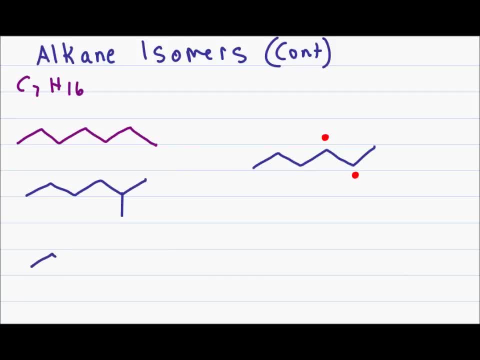 So I have 2-methylhexane and 3-methylhexane For the 5-carbon chain. I get two substituents. I can put them together or separately, So it can have on 2 and 3, I can have them on 2 and 4, or it can have them together on. 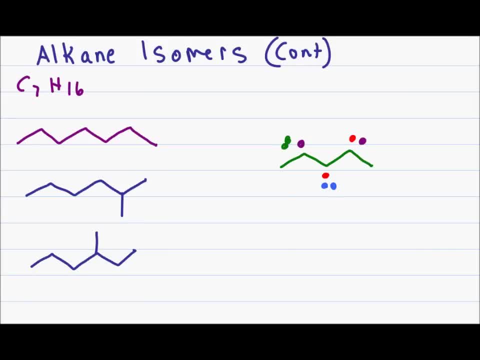 2 or together on 3.. Remember, together on 4 is the same as together on 2.. For the first one, I put my substituents together on the second carbon, giving me 2, 2-dimethylpentane. 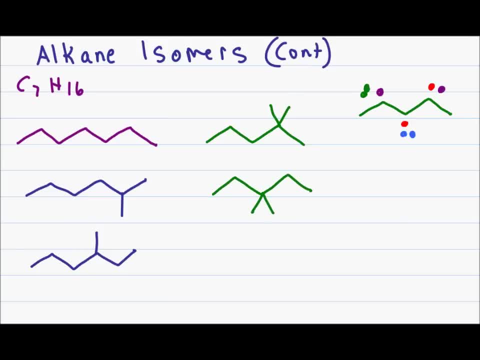 For the second one, I will have 3, 3-dimethylpentane. Then I will separate them to give me 2, 3-dimethylpentane. I'm going to squeeze this one in here for 2, 4-dimethylpentane. 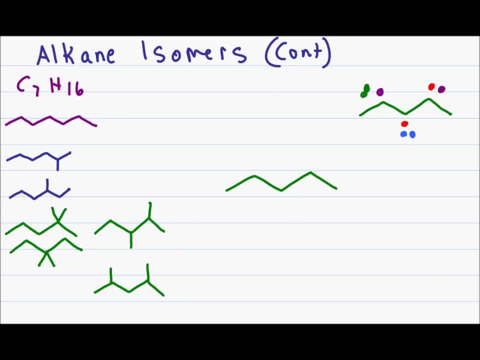 And lastly, on a 5-carbon chain, I can also do an ethyl substituent, since it won't have. it won't extend the length of the chain. No matter how I count it, I hit three at the center. 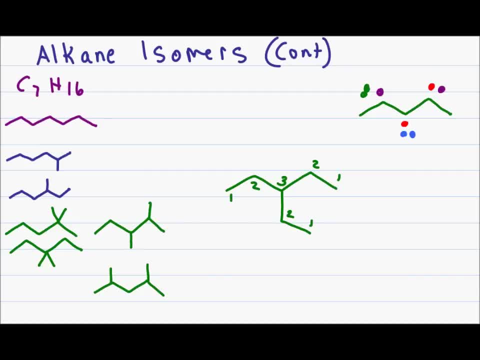 which means that it'll be three ethyl pentane On a four carbon chain. I get three substituents and I can only put them as methyl substituents. If I do an ethyl, then I actually extend the length of the chain, giving me one, two, three, four, five, which is longer than the parent chain.